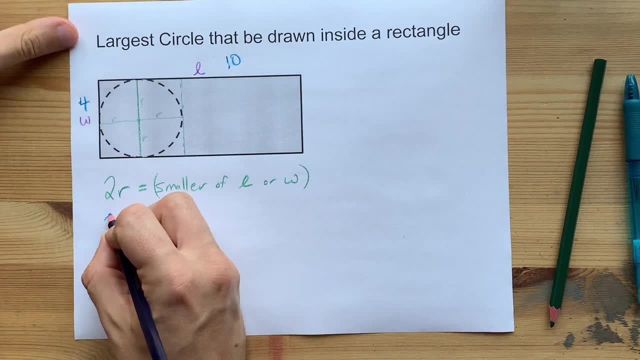 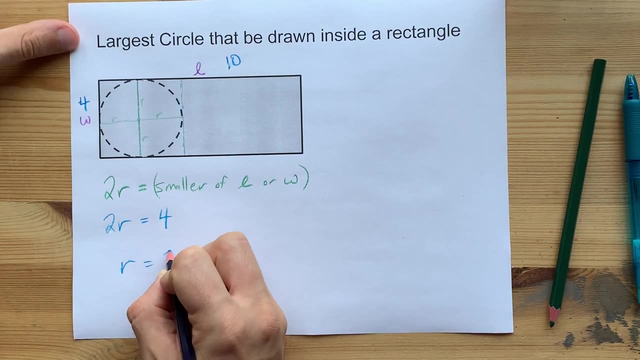 over here that you're never going to use. So the point there is that 2r would equal the 4, the smaller of the two dimensions, and the r would be 2.. I don't know centimeters, inches. 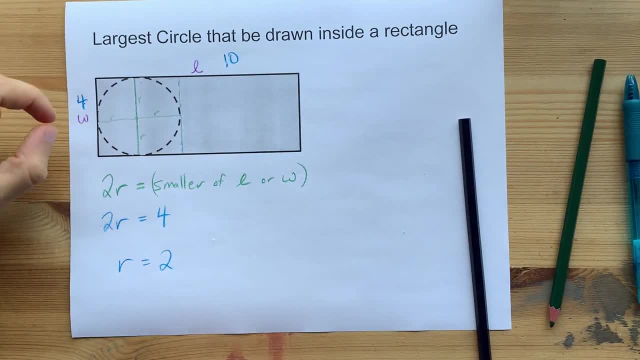 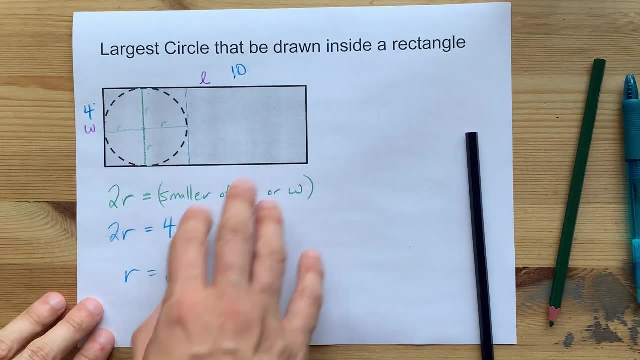 whatever, The circle can't get any larger than that, or it would be wider than the width of this rectangle itself. Ah, pretty straightforward. Hopefully it helped you visualize. Best of luck. 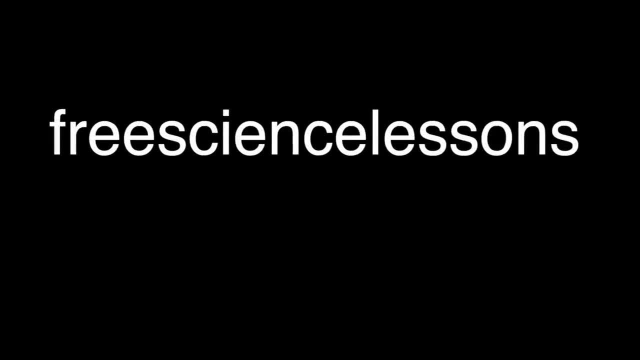 Hi and welcome back to freesciencelessonscouk. By the end of this video, you should be able to describe the roles of the different tissues in a plant. Now I need to be clear here. there's a lot of detail in this video and the best thing you can do is learn it. It's very likely to be on your 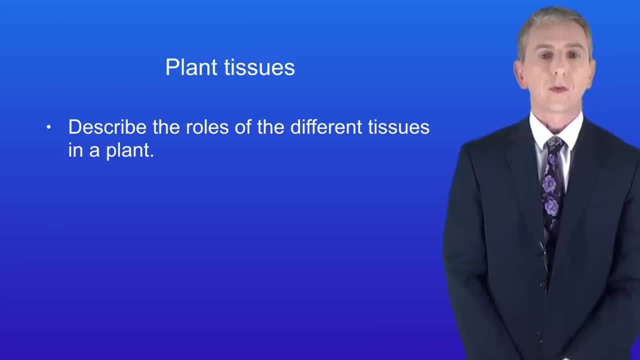 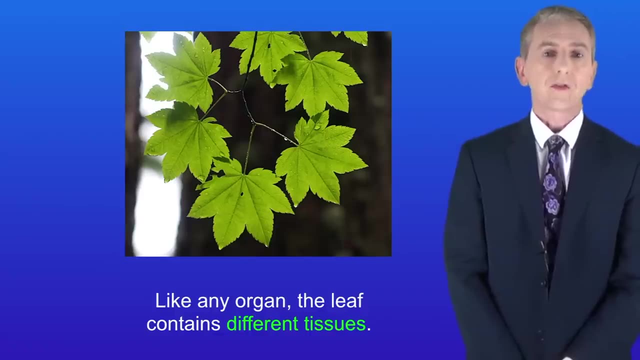 exam. In the last few videos we've been looking at photosynthesis. Remember that photosynthesis takes place in leaves. The leaf is a plant organ. Like any organ, the leaf contains different tissues. We'll be looking at the functions of these tissues in this video. This diagram shows you a cross. 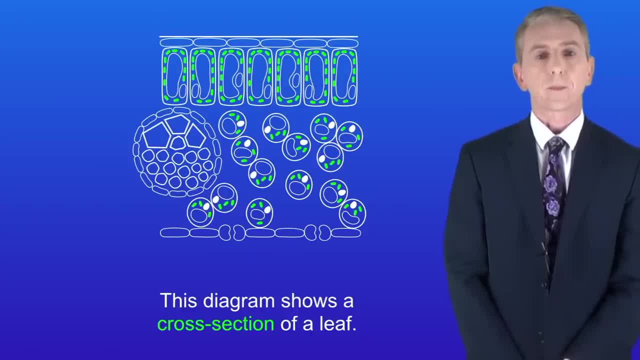 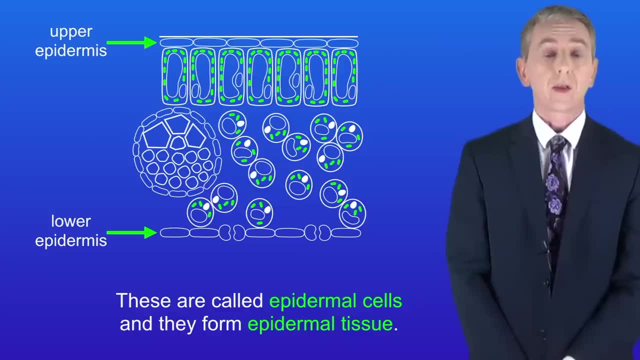 section of a leaf. In other words, the leaf's been sliced from top to bottom. The top and bottom of the leaf are covered with a layer of very thin cells. These are called epidermal cells and they form epidermal tissue. So at the top of the leaf we've got the upper epidermis and at the bottom 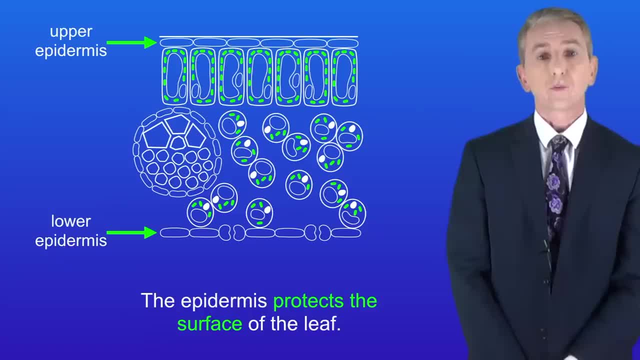 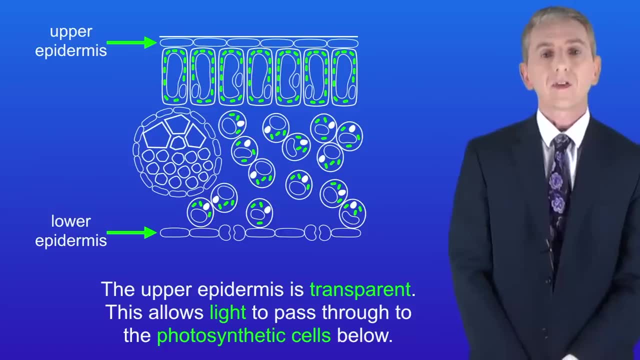 of the leaf. we've got the lower epidermis. The epidermis protects the surface of the leaf. Now the key adaptation of the upper epidermis is that it's transparent. This allows light to pass through to the photosynthetic cells below.